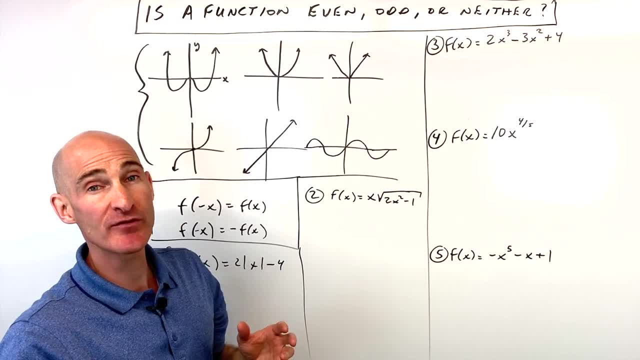 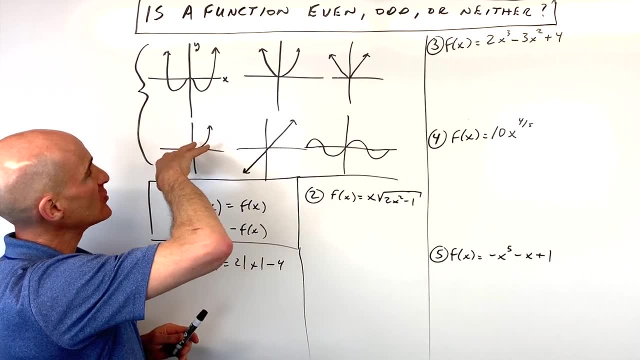 It's even So. all three of these top ones are going to be even functions. Reflection over the y-axis: that's how you test With odd functions. you want to see if it's 180 degree like a half turn rotation about the origin: 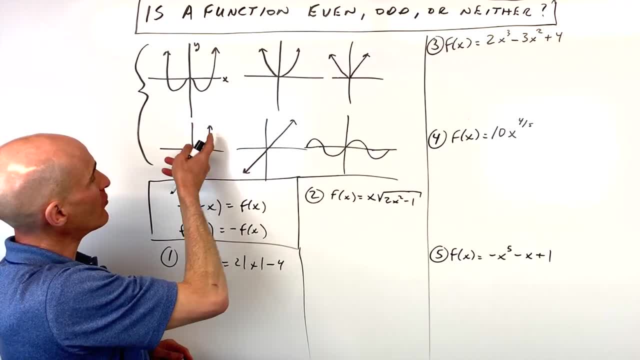 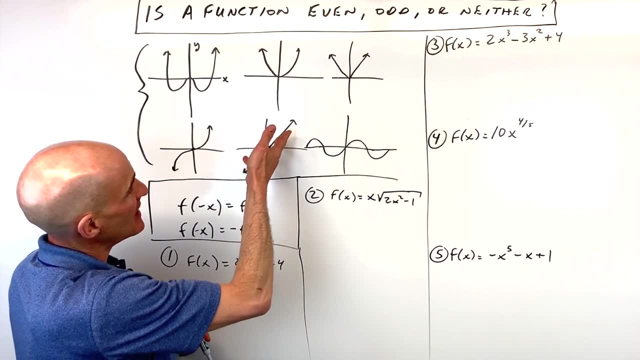 If you rotate this y equals x cube graph around the origin 180 degrees, it will match with itself. That tells us that it's an odd function. For this one, this is like the line y equals x. Again, if you take this graph and you rotate 180 degrees a half turn, it will match with itself. 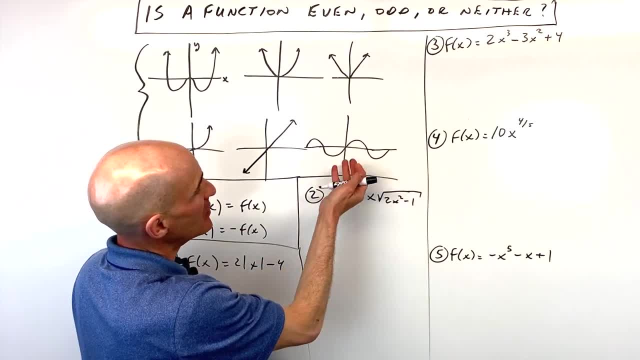 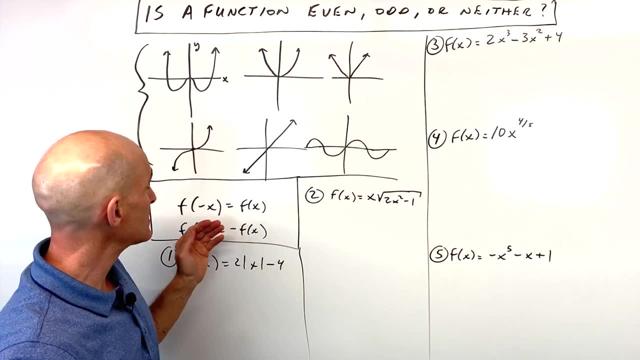 That means it's odd. And this one's like: a y equals sine of x. And again you can see: if you rotate it 180 degrees it matches with itself. So these are going to be odd functions. But algebraically the way you test it is you put negative x into your function. 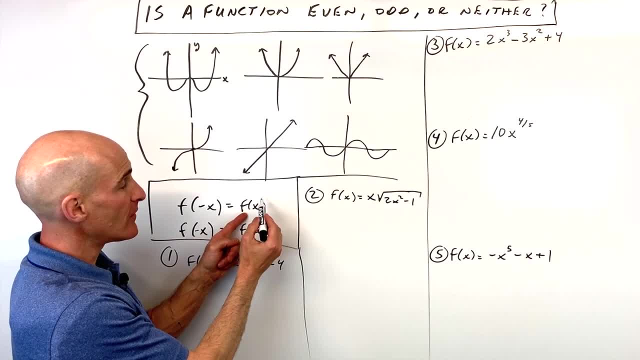 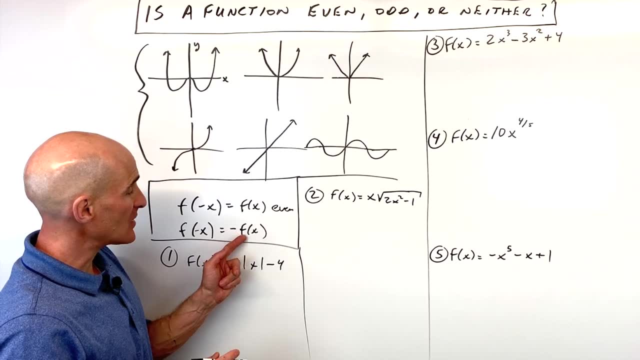 okay, in place of x on the right side. If you get the original function back, then we call this an even function, Meaning if you graph it, it's going to be reflection over the y-axis. If you put negative x in and you get the original function back, but it's multiplied by negative one. 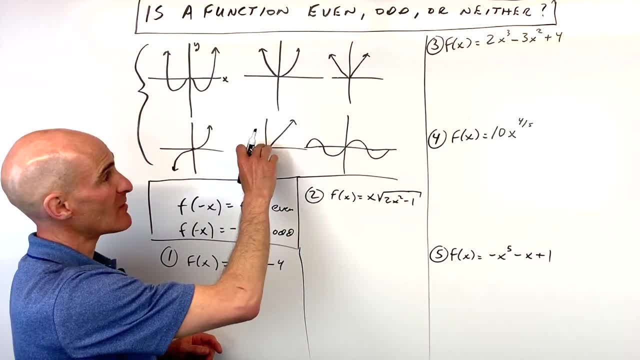 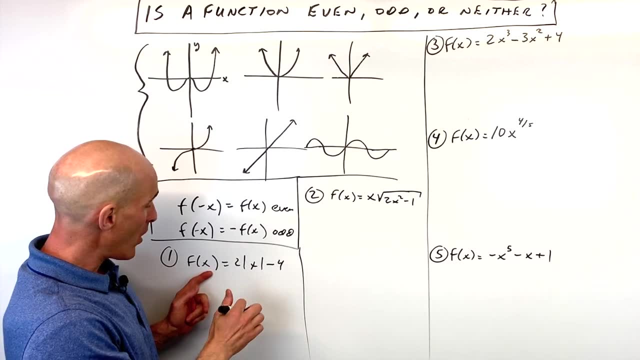 then that means that it's an odd function, which means it's a rotation about the origin, like these bottom three ones here. So let's go through some examples. These are some typical ones that you'll see in your class. For number one, f of x equals two times the absolute value of x minus four. 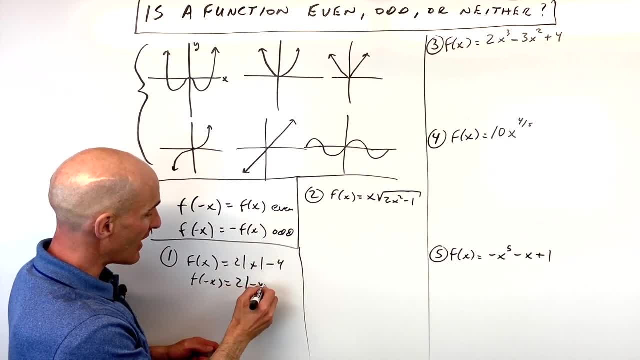 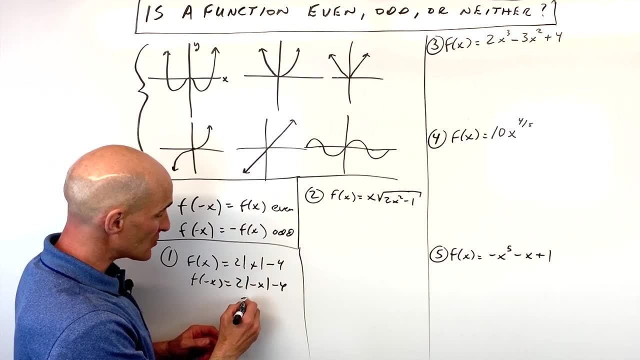 So our test is: we're going to put negative x in in place of x. We know when you take the absolute value of a negative quantity or a positive quantity, you end up getting that positive quantity. So this is really going to be the same as two times absolute value of x minus four. 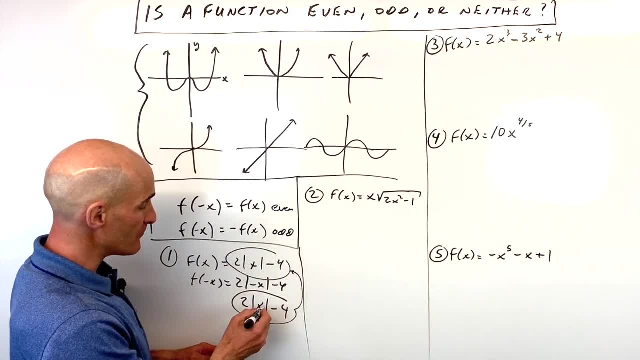 You can see, we're getting the absolute value of x minus four. We're getting back the original function, the original equation, When we plugged in that negative x. that tells us that this is going to be an even function. Okay, let's look at number two. 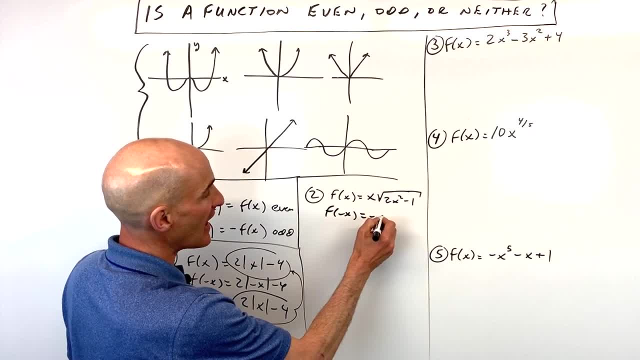 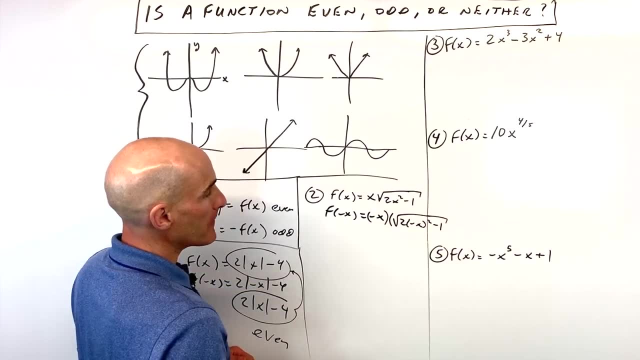 This one here again, same process. All you're doing is, wherever you see x, just put negative x in. So this is going to be two times negative x squared minus one. But when you have a negative squared, that's going to be the same thing as a positive right. 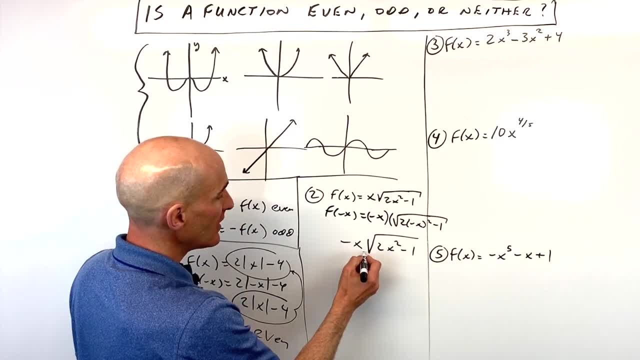 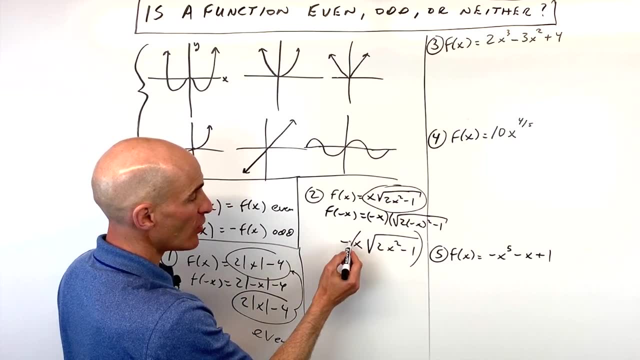 It's got a negative times a negative is a positive. So that's the same as two x squared minus one times zero Negative x. Now you can see this whole equation here. It's just like the original function we had. It's just now. it's multiplied by negative one. 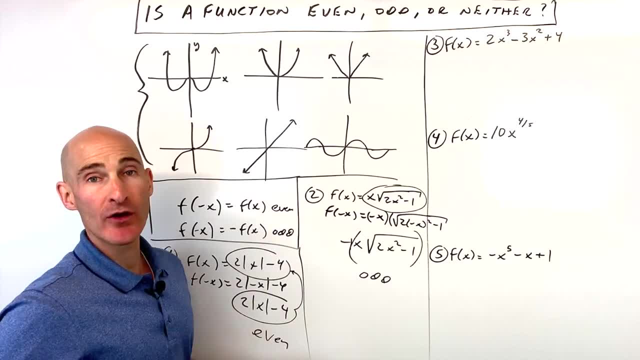 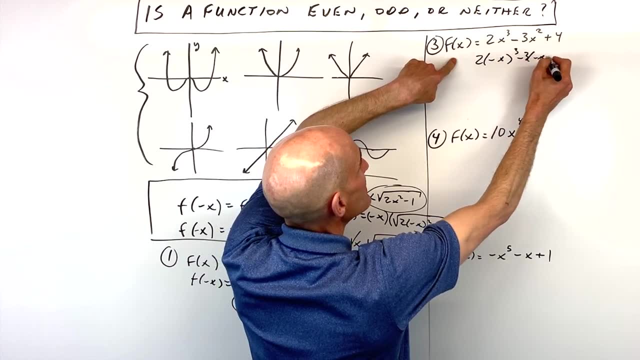 And that tells us that it's an odd function, Meaning it's going to be a rotation around the origin. Okay, number three, same idea. We're just going to replace x with negative x. Wherever you see that x, put in negative x. 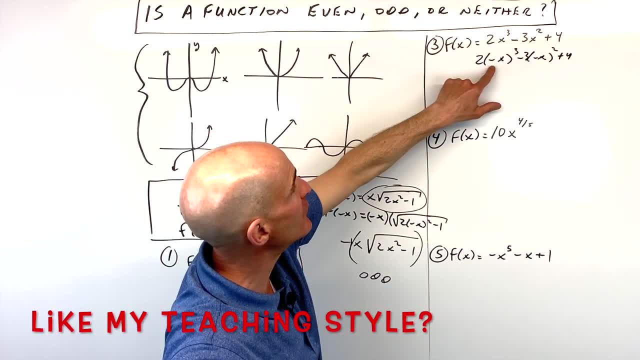 And the key is to put it in parentheses So you take it as a group. But if you have a negative to an odd power, that's going to make it negative. If you have a negative to an even power, that's going to make this quantity pi. 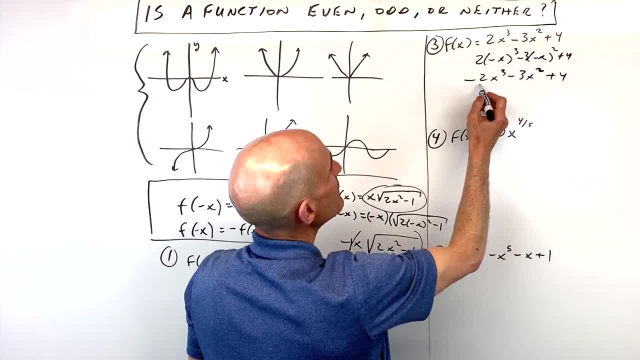 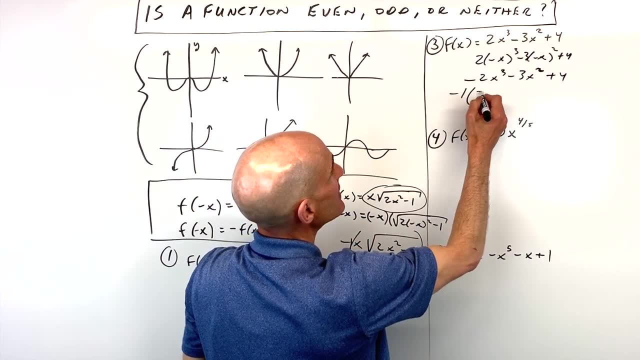 That's going to be a positive. But then times negative three, of course, is negative. When we look at this, is it the same as the original function? Definitely not. If we factor out a negative one like this, we get two x cubed plus three x squared minus four. 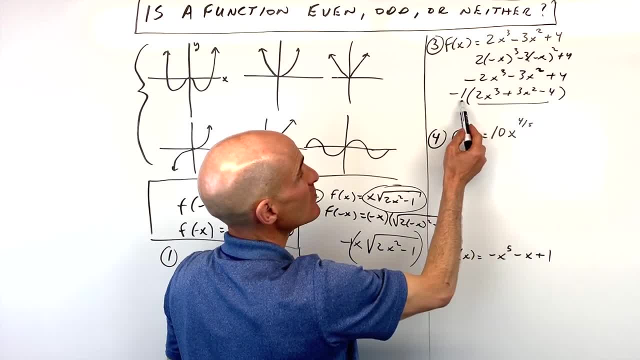 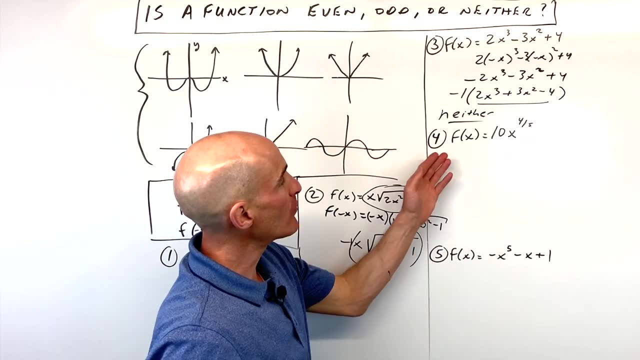 Does this look like the original equation? No, it doesn't. If it did, and it was just multiplied by negative one, that would be odd. This one is actually neither even or odd. Okay, for number four. we've got some fractional exponents, rational exponents. 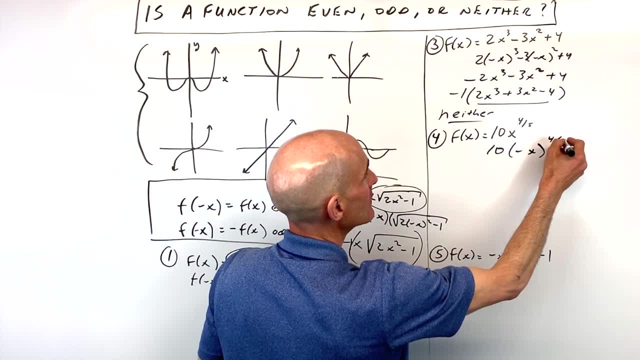 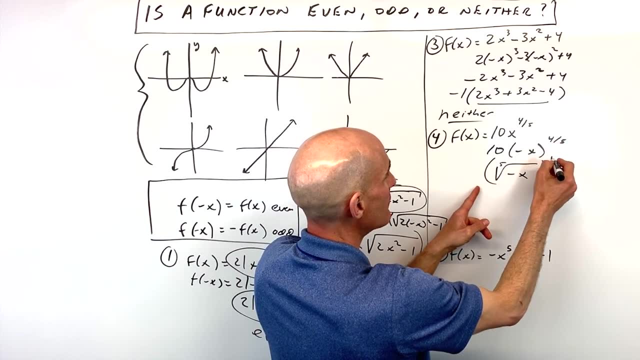 Same process. We're replacing x with negative x. right, And remember to switch this into radical form. the denominator is the root, The numerator is the power. But think about it When you have a cube root or the fifth root or the seventh root of a negative number. 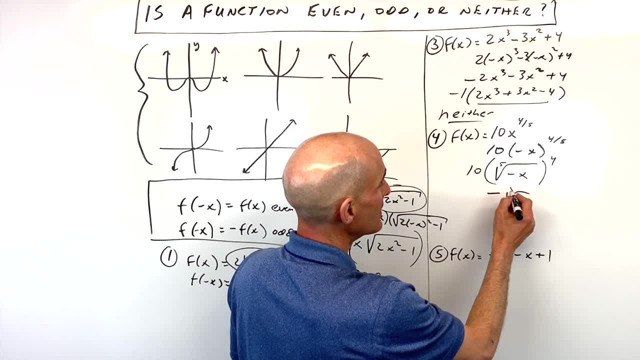 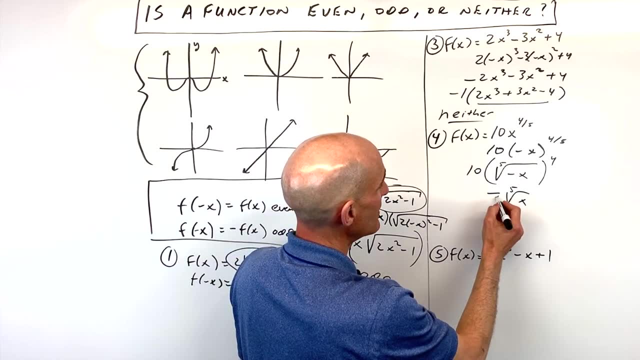 that's just going to be the same as negative. whatever this quantity is here right? So like if you had the cube root of negative eight, that's just going to be negative. two, It's going to be a negative number, And then multiplied by this ten here, this is going to make this a negative ten. 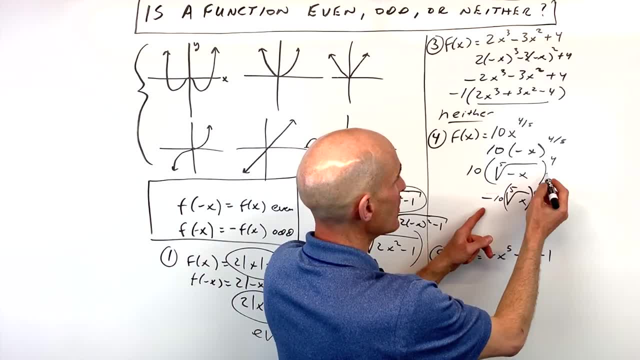 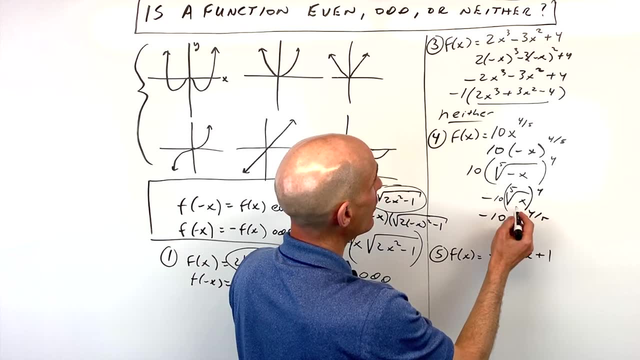 Okay, let me just move this down here. negative ten: This quantity here is raised to the fourth power, right? So you can see we're ending up with negative ten times x to the fourth-fifth power. It's the same as the original function, but see how it's multiplied by negative one. 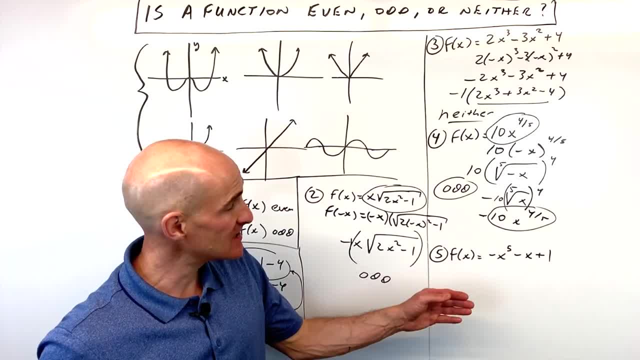 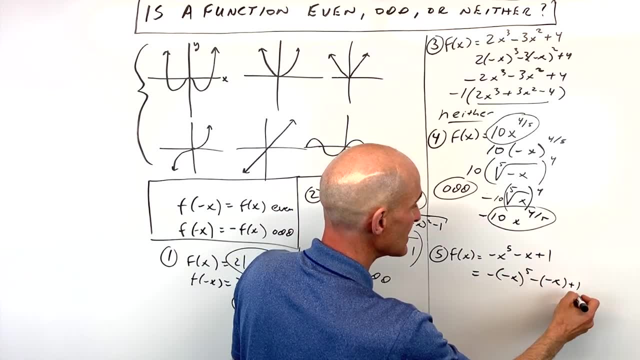 That means this is going to be an odd function. And then the last example, number five, same process. We're replacing x with negative x. Again, notice how I'm putting it in parentheses, to keep everything organized. Negative to an odd power is going to be negative, so this is just going to be like that.